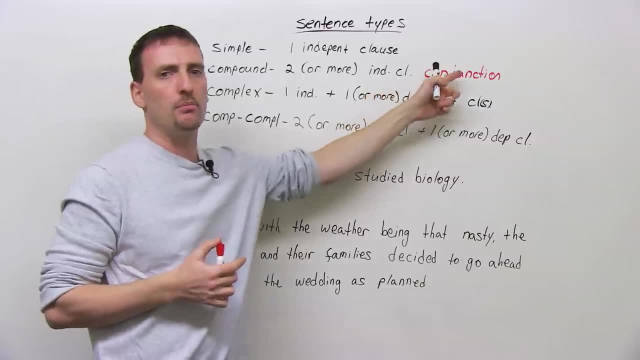 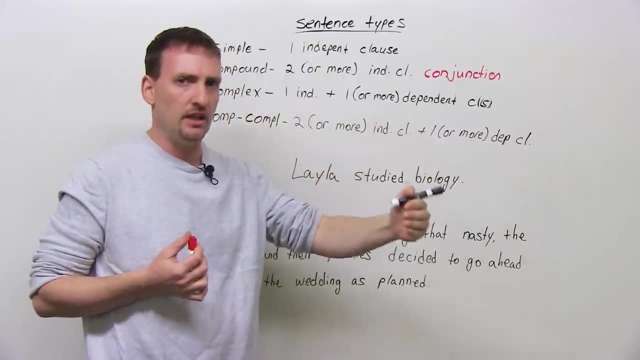 So We join two independent clauses with a compound conjunction. You can have more, but again, you have to be a little bit careful. Once you get to three, start to look for a way to finish your sentence, because if you get to the fourth you already have a crazy sentence. 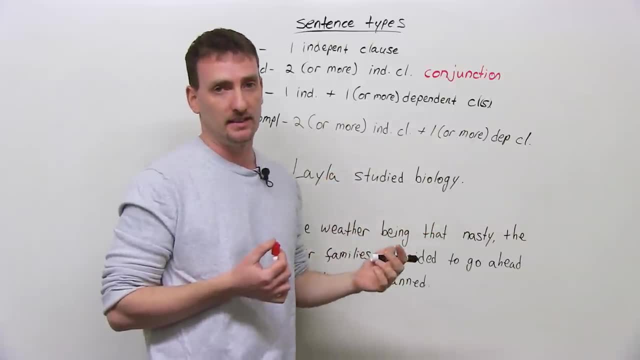 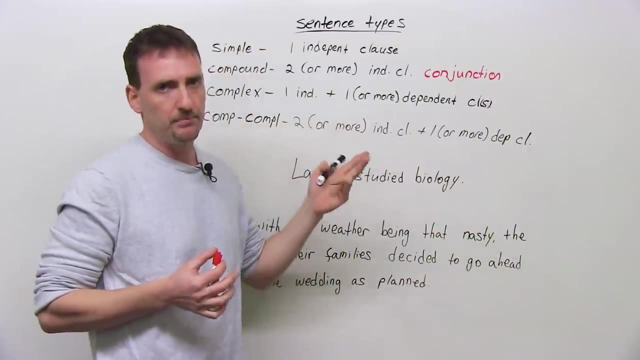 that has the Runs, the risk of being a run-on sentence. Eventually, you're going to make a mistake, you're going to miss something and the whole sentence falls apart. I don't recommend three, but you can put three, Then we have. 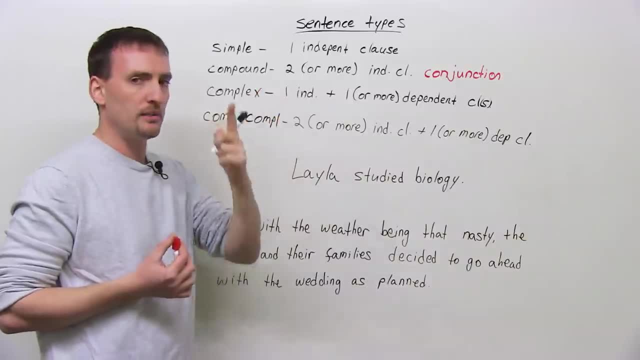 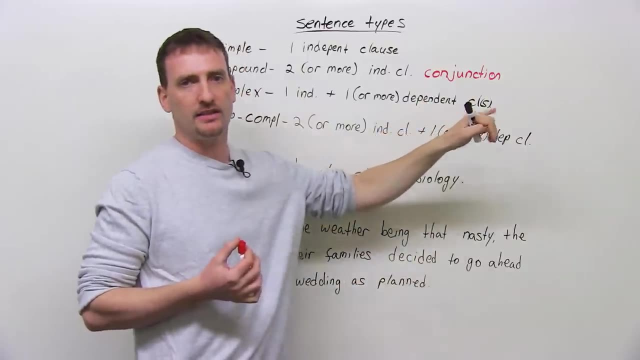 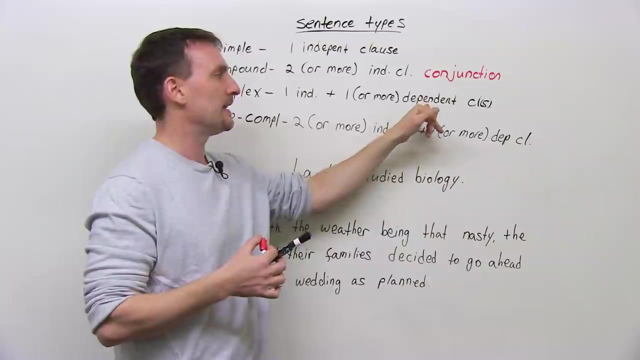 Then we have a complex sentence. A complex sentence has one independent clause plus one or more dependent clause. A dependent clause is a clause that has a subject and a verb but cannot stand by itself. It is not a complete idea. It has some sort of relationship to 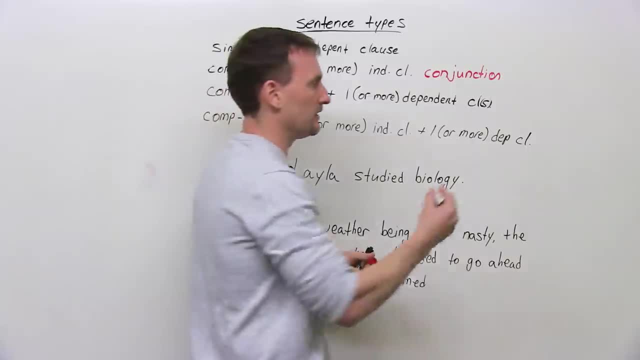 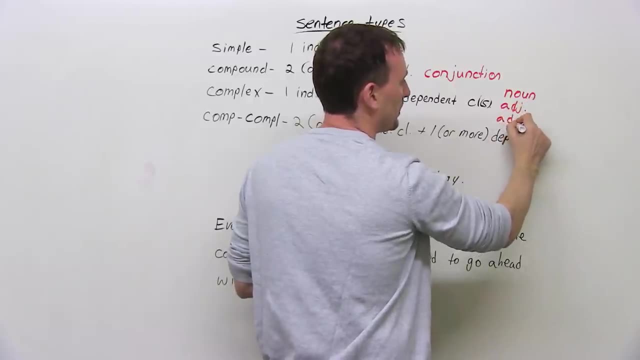 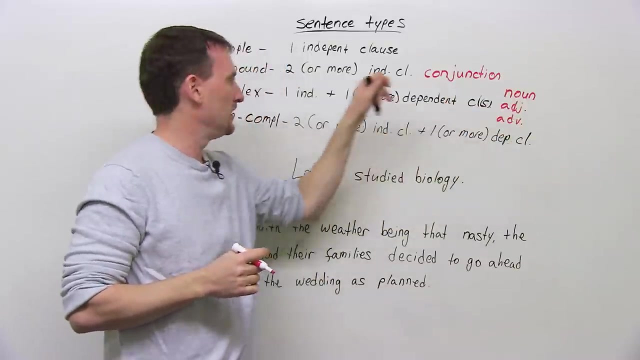 the independent clause. We have three types of dependent clauses. We have noun clauses, we have adjective clauses, we have adverb clauses. Okay, That's a whole separate lesson. you can look at that later. but you have to have one of these plus one of these and you have a complex sentence. 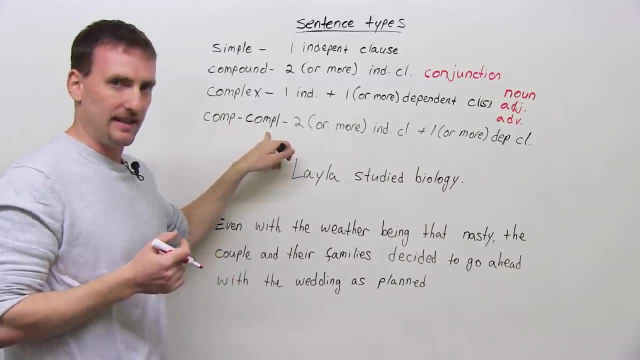 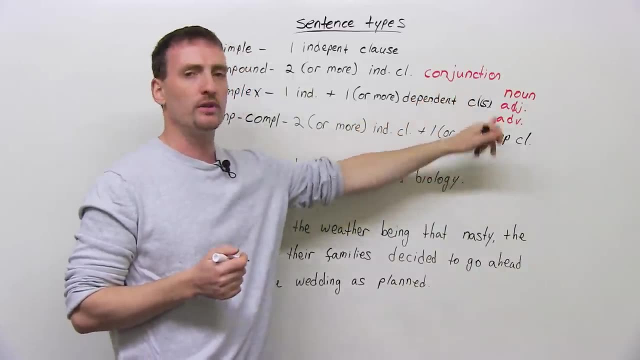 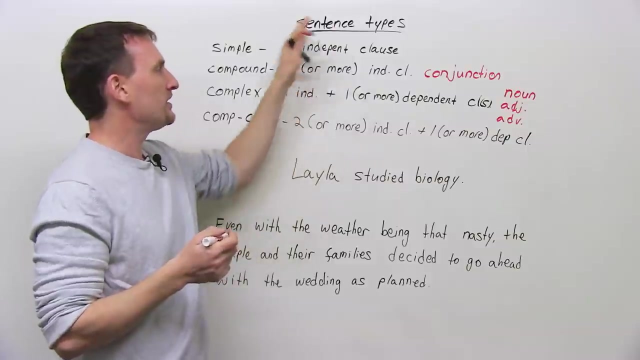 Next we have a compound, complex sentence. Here you have two or more independent clauses, again joined by a conjunction, and one or more dependent clause. Okay, So you have basically all the elements in this sentence. Then, once you have all this stuff, you can add as many. 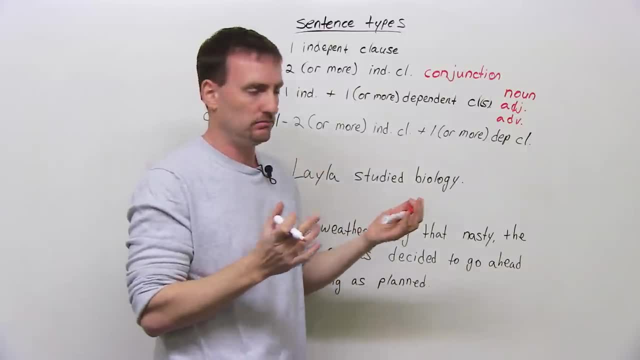 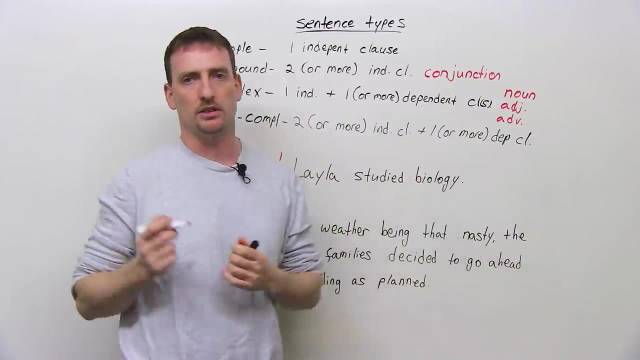 complements or basically extras, as you want. So let's look at an example. We're going to start with the simple sentence: Leila studied biology. Very simple: I have a subject, I have a verb, I have an object. 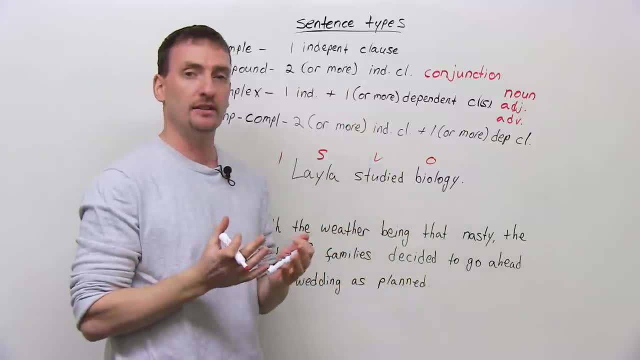 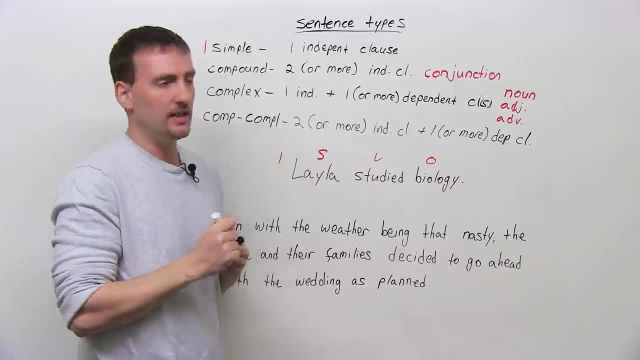 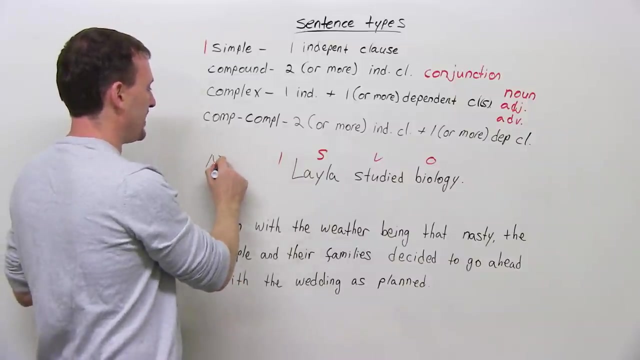 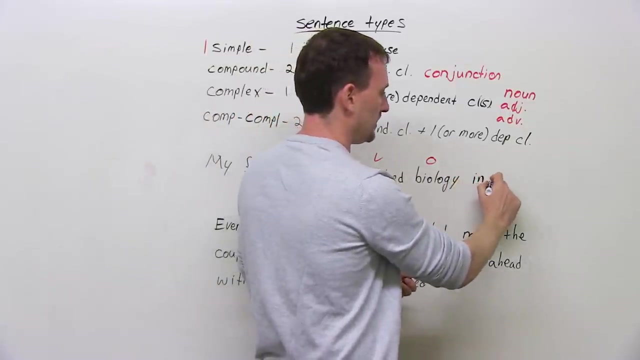 Okay, This is a simple sentence. it's an independent clause. it can stand by itself. it's a complete idea. Now I can add anything I want to this. that is not another clause of any type and it'll still be a simple sentence. So I can say: my friend Leila studied biology in university. 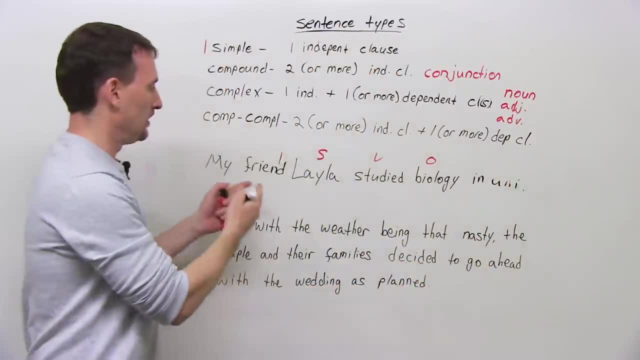 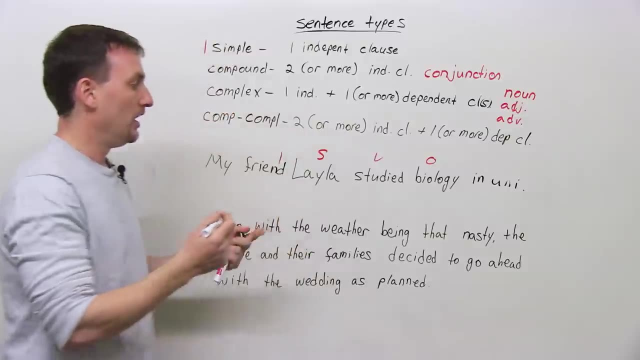 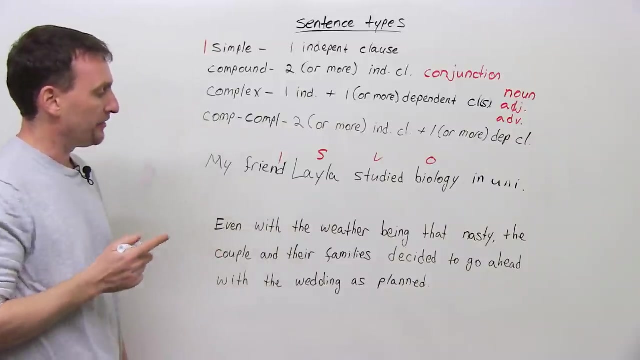 I'll just say uni for short. I have more information, but do I have a different type of sentence? No, it's still a simple sentence. Now let's look at this First. let me read it to you. Even with the weather being that nasty, the couple and their families decided to go ahead. 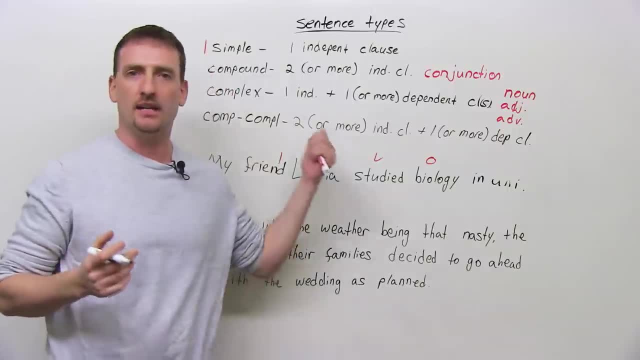 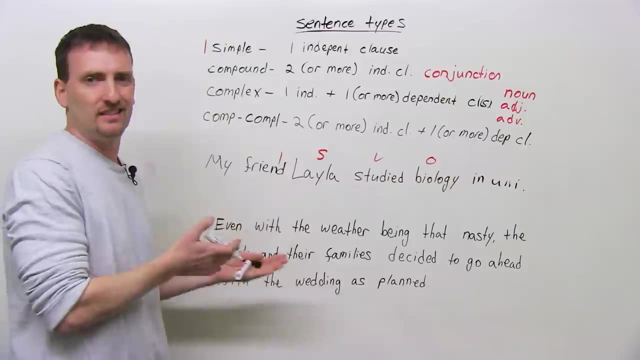 with the wedding as planned. Now you're thinking, wow, that's got to be a complex sentence, right? It's so long, There's so much information in it, But if we look at it carefully, it is still a simple sentence. 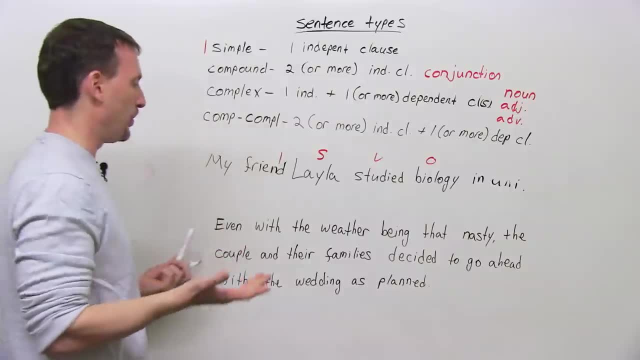 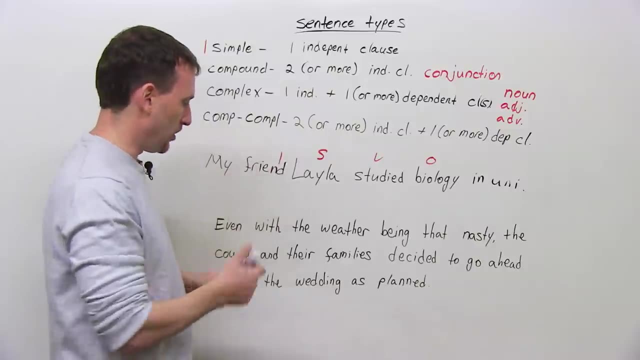 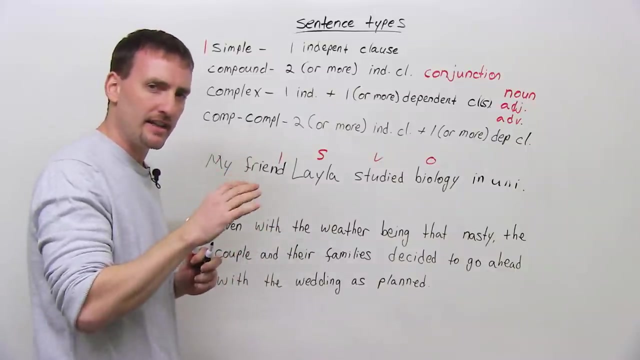 Why? Because we only have one independent clause. Where is it? Well, find the subject and verb combination, Okay, First. so what is the subject in this sentence? Give you a few seconds, figure it out. Hit the pause key, look at it. Okay, we're back. Here's the subject: The couple and their families. 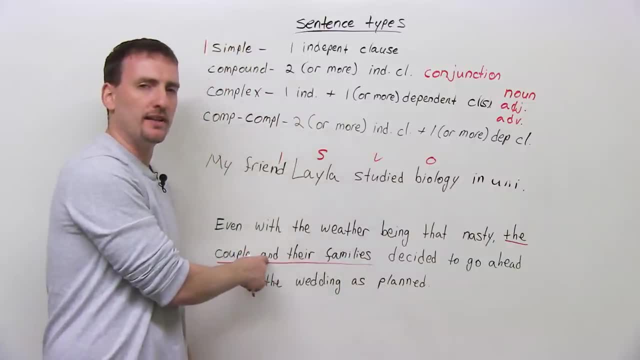 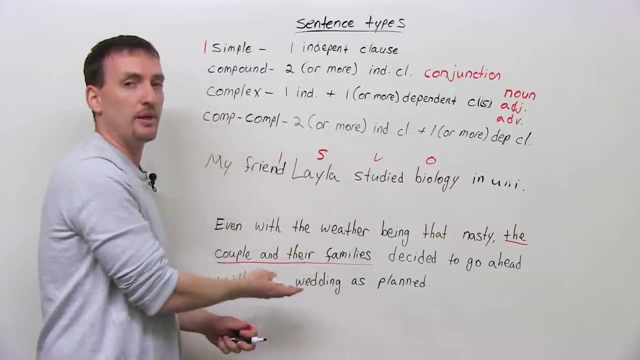 Now don't get confused. with this end. This is not joining another clause to another clause, This is just joining one part of the subject to another part of the subject. So here we have a compound subject, not a compound sentence. So one subject. 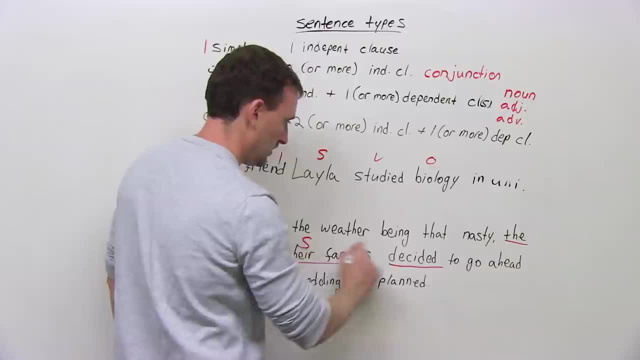 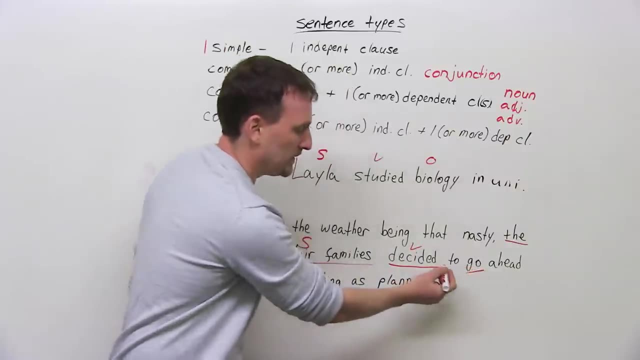 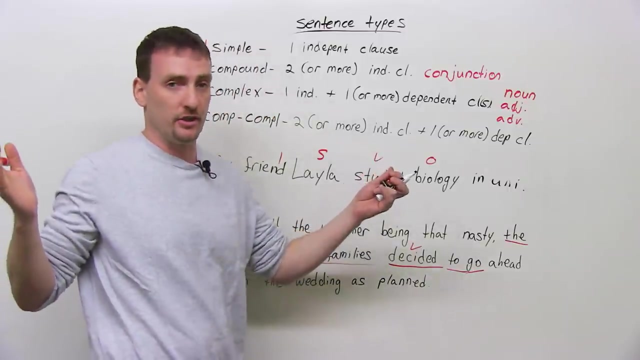 Decided Subject verb. Do I have any other subjects and verbs? Do I have any other verbs? I have this verb, but this is an infinitive verb. Right A clause only has one tense verb. You can have ten verbs in a sentence, but only one will be the tense verb in the independent. 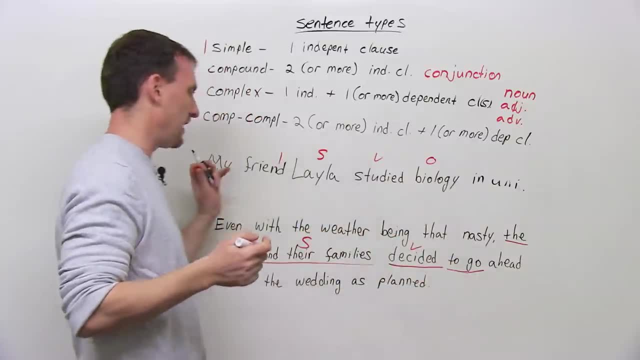 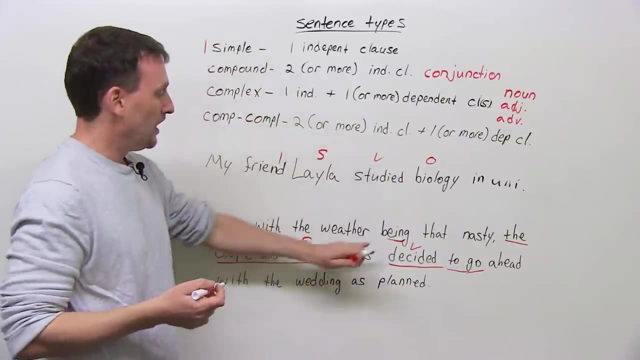 clause And what goes with this? Nothing, Okay, Oh, here's another verb, but it's not really a verb, It's a participle. Okay, So now here's my subject, here's my verb, here's my object. This whole thing is the. 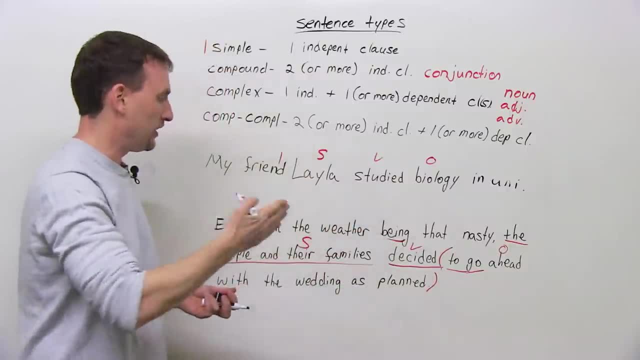 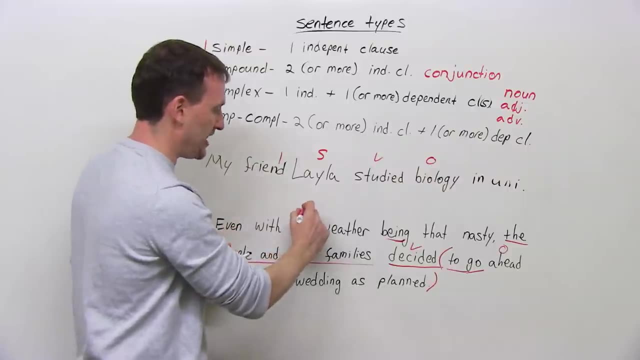 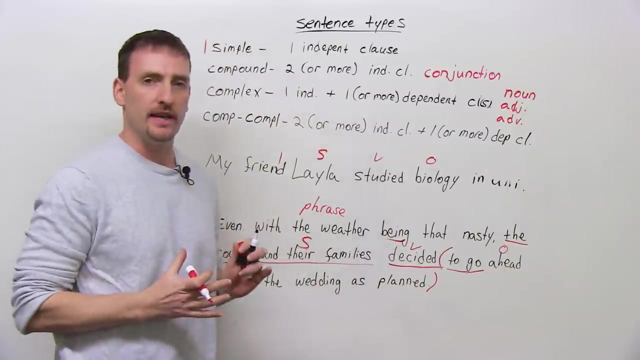 object to decide. It decided what: To go ahead with the wedding as planned, Even with the weather being that nasty. So all of this is what. This is a phrase. It does not contain a subject. it does not contain a verb, Right? So here I have a simple sentence with lots. 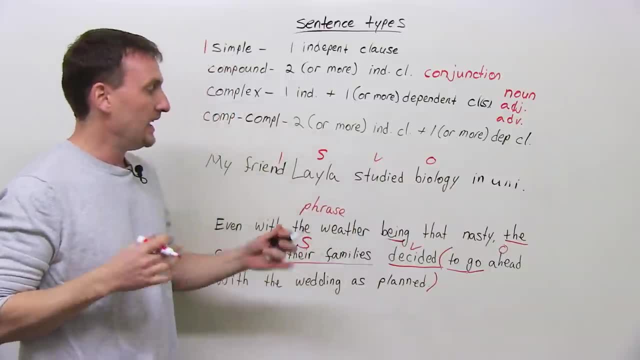 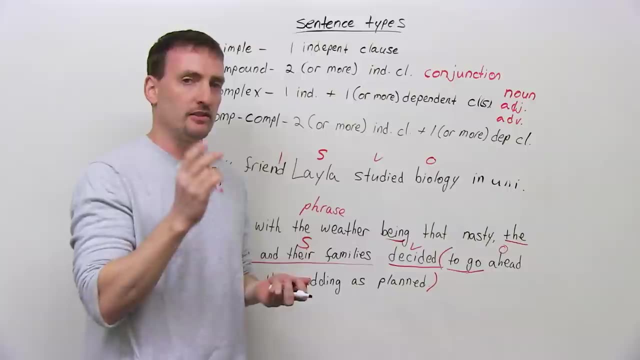 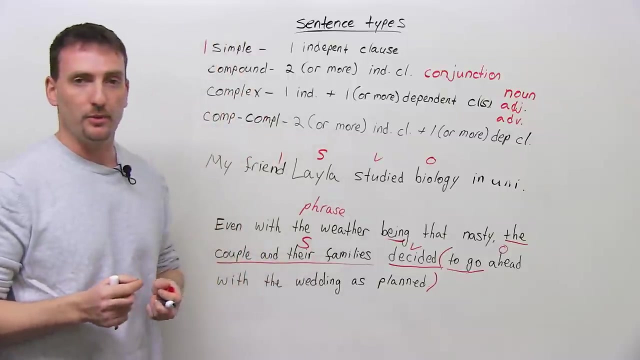 of additions to it. Okay, Very simple. The key is to recognize what's involved in the sentence. You can have a very long sentence As long as it only has one subject-verb combination. it is a simple sentence. Okay, Let's look at a few of the other ones now and see how they work. 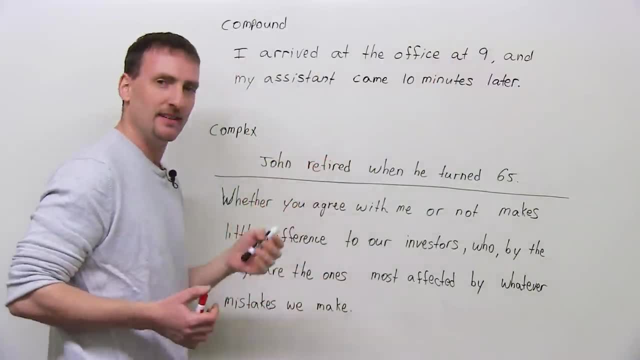 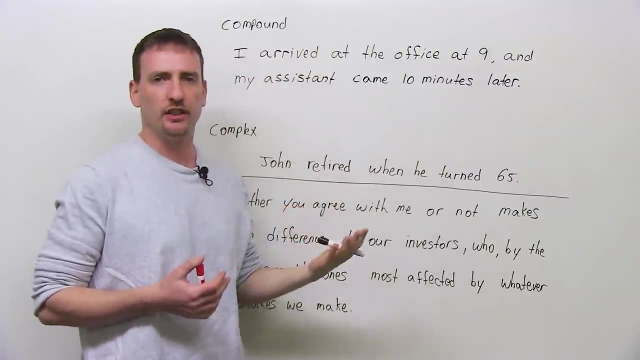 Okay, so we're back. Let's look at the next set of examples. Let's look at compound sentences. Compound sentences- I only gave you one example here, because it's very straightforward: Have your independent clause, have your compound conjunction, have another independent clause. 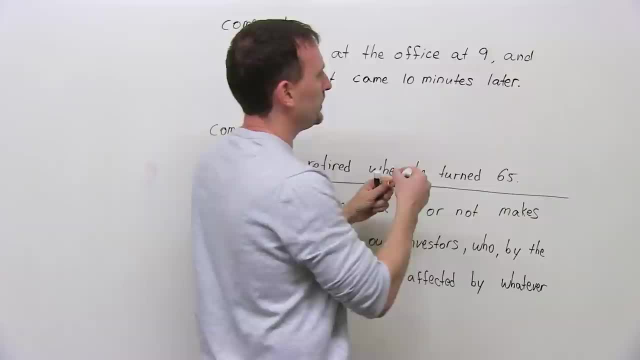 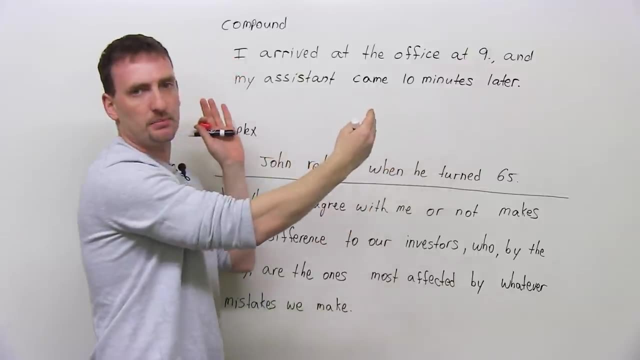 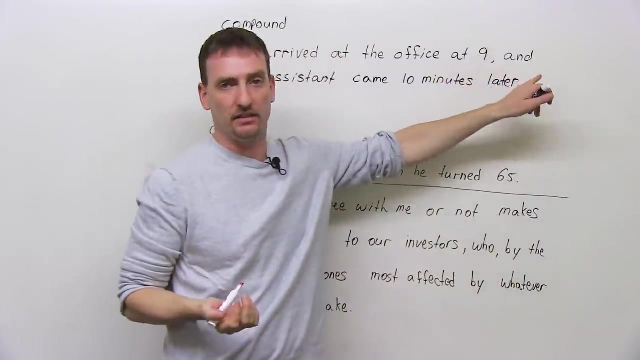 I arrived at the office at 9.. I could put a period here And that's a complete sentence. My assistant came 10 minutes later. This is a complete sentence. Two independent clauses. All I'm doing is joining them with the conjunction end. But remember I said you can have one. 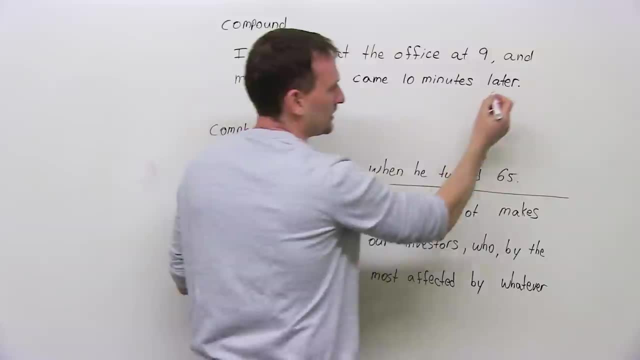 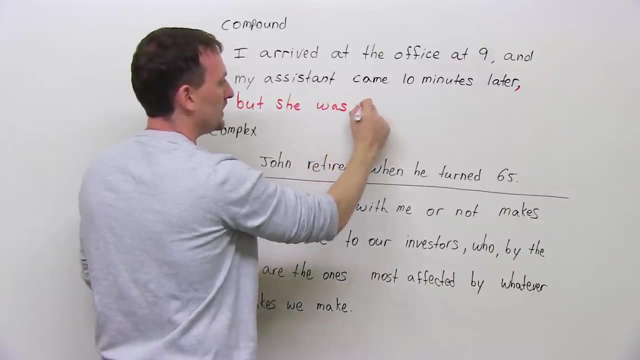 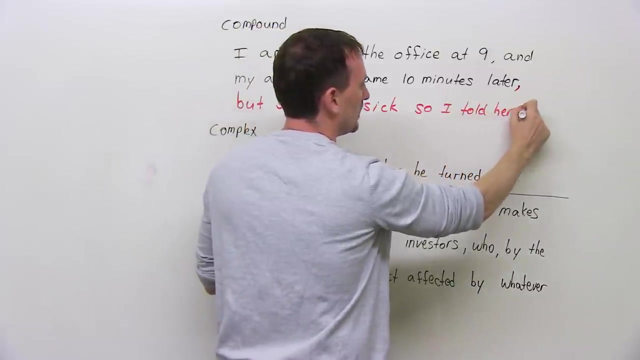 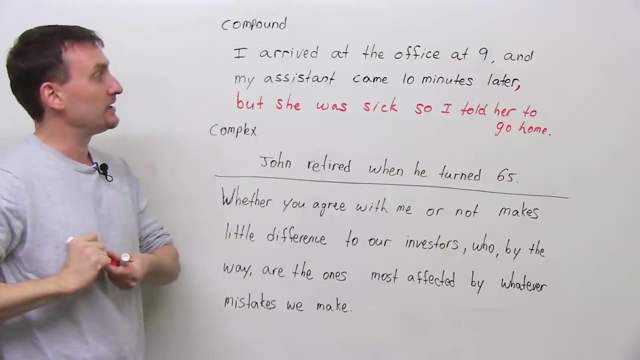 you can have two. you can have three independent clauses. I can add another one. All right, Okay, another one, But she was sick, so I told her to go home. Now. I arrived at the office at 9, and my assistant came 10 minutes later, but she was sick, so I told her to go home. 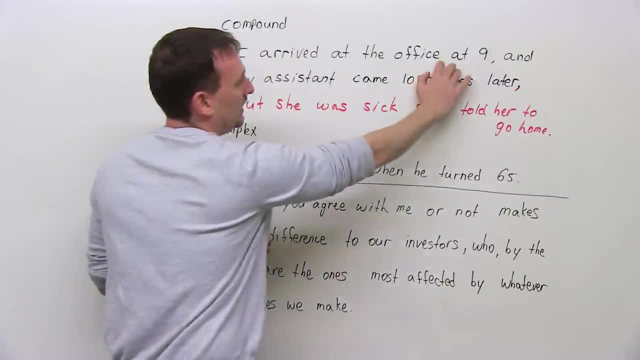 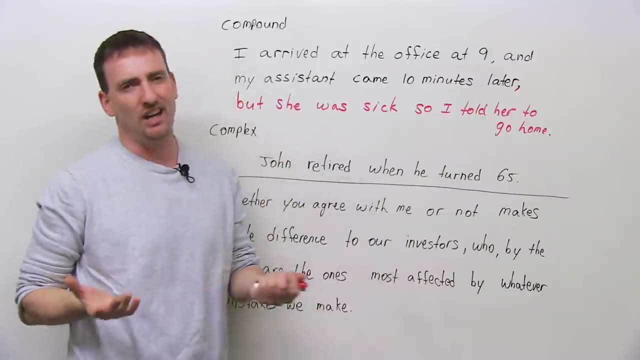 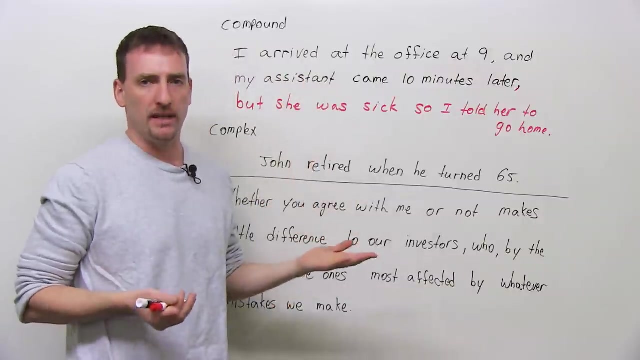 How many independent clauses do you count here? One, two, three, four. Now is this a good sentence? No, it's not. Is it grammatically correct? Yes, it is. So this is okay, but I wouldn't recommend it. I would split this into two sentences. I would put a period here. 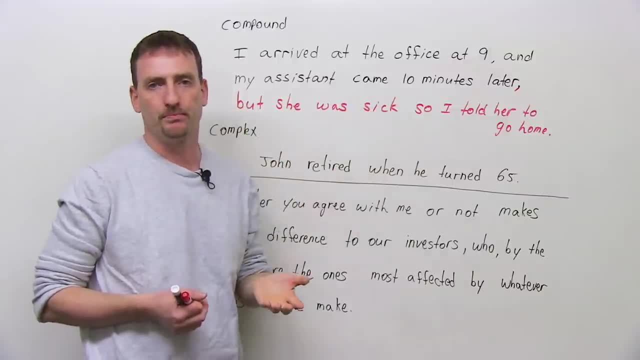 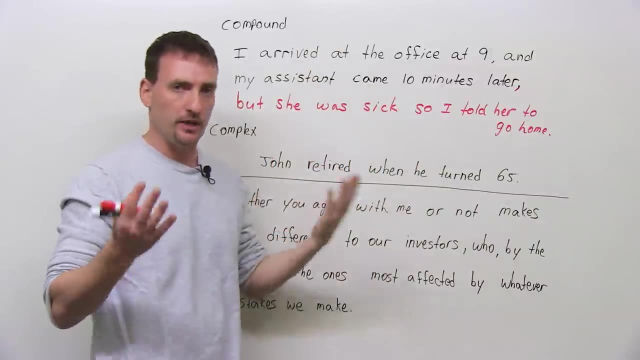 I would take out the, but I would say she was sick so I told her to go home. I'll just make it a whole: two separate ideas instead of one One joined idea. But again, that's up to you. I don't recommend it, but it's grammatically. 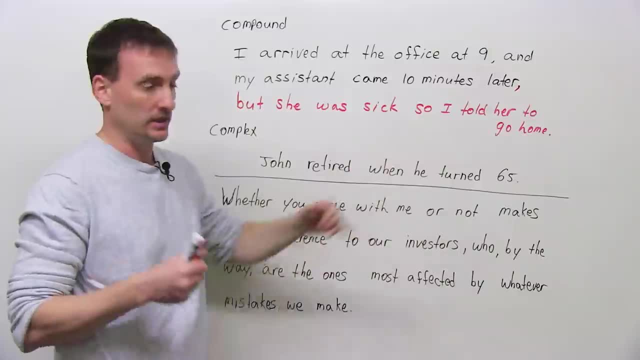 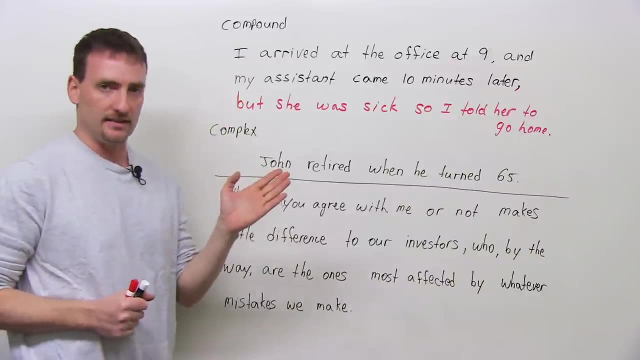 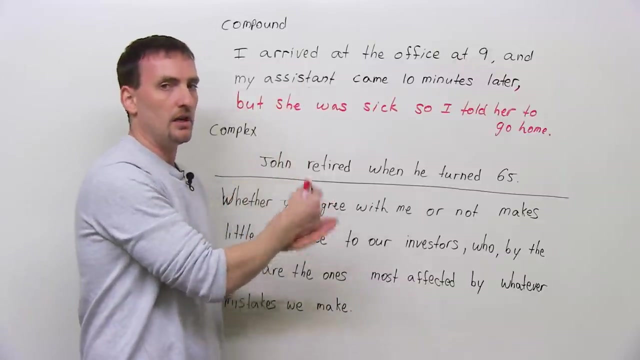 okay, So it's also a conjunction. It is not an adverb conjunction, it is a compound conjunction. Next, let's look at complex sentences and this is where people start getting a little bit scared. but you don't need to be. Just remember: independent clause, dependent clause. 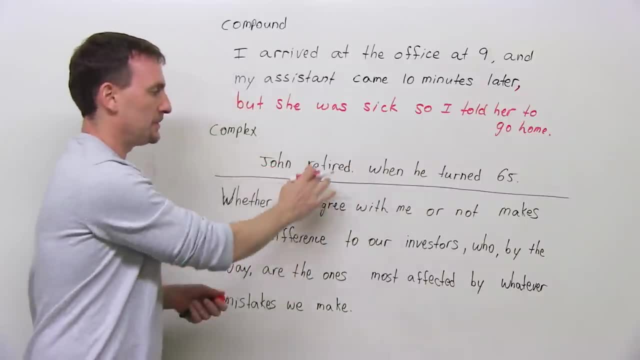 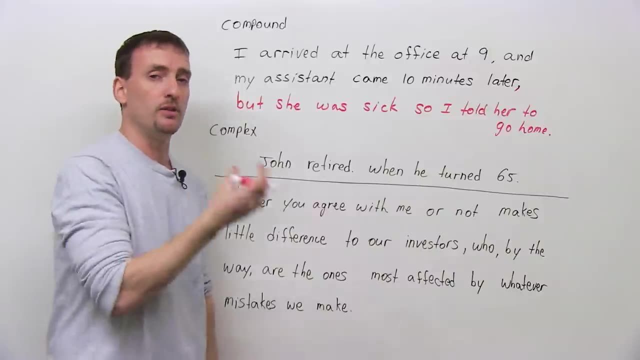 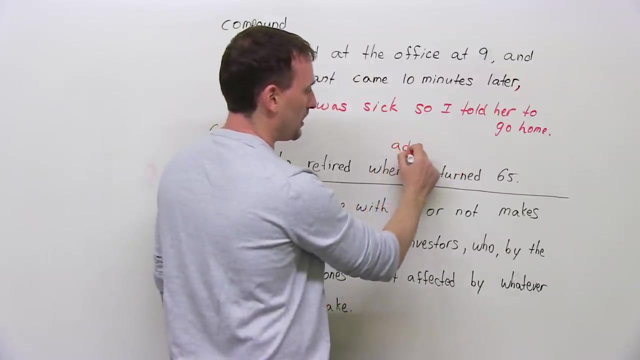 John retired. John is a subject. retired is a verb. I have a complete idea. That's all I need to know. He doesn't work anymore. but I want to give you more information. John retired when he turned 65. So this is an adverb clause. 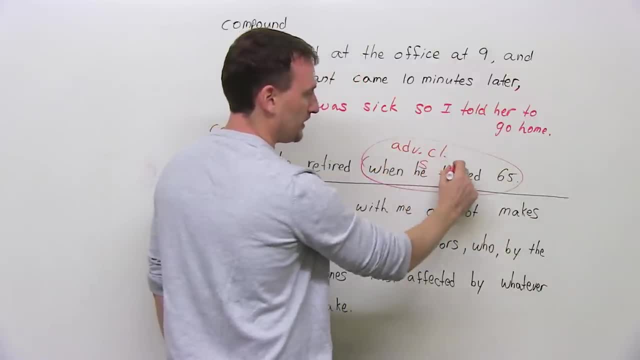 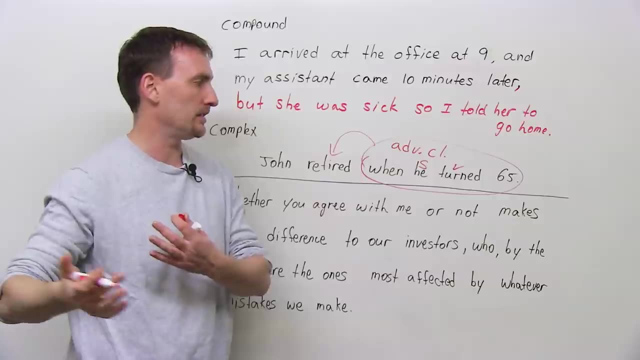 Okay, This whole thing is an adverb clause, It has its own subject and verb and it tells you something about the verb retired. When did he retire? When he was, When he turned 65. Turned means had his birthday, Okay. 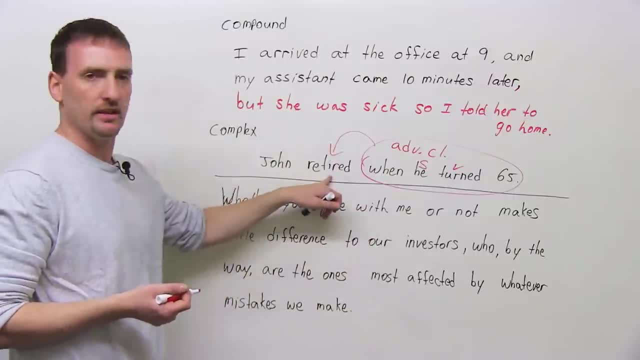 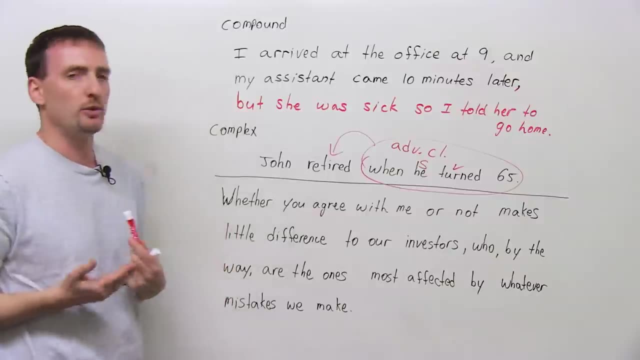 So this is Again. this is a complex sentence. It's much longer than this one, but it works in the same way. Let me read it to you. "whether you agree with me or not makes little difference to our investors who by 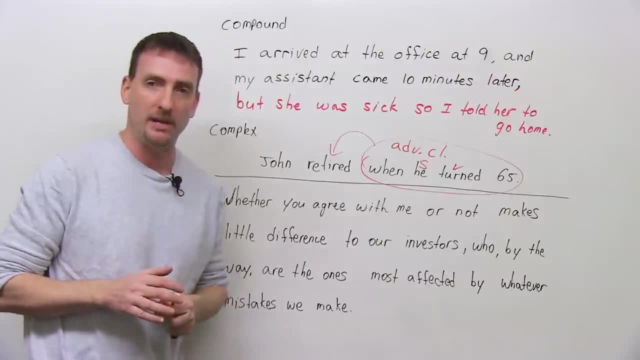 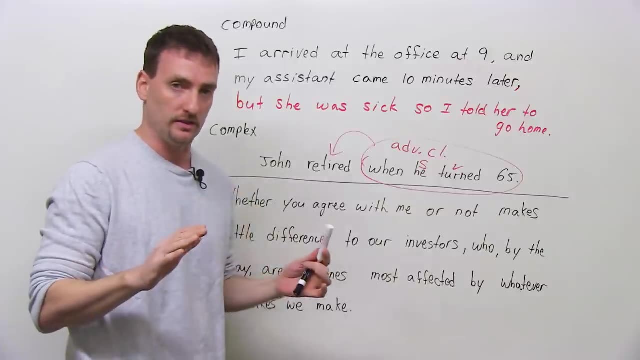 the way, are the ones most affected by whatever mistakes we make". Now you're thinking: well, that's a crazy sentence. Where do I start? Start with the independent clause. always A little bit trickier here, though, Okay, The easiest way to find. 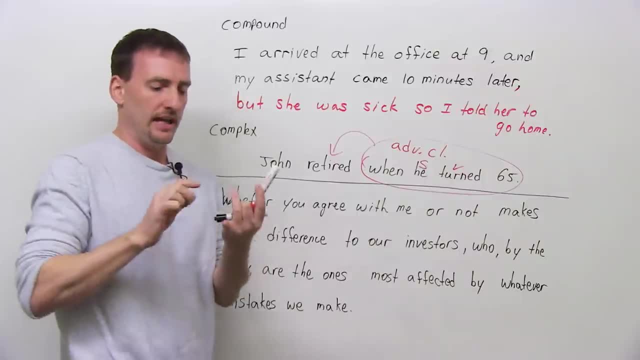 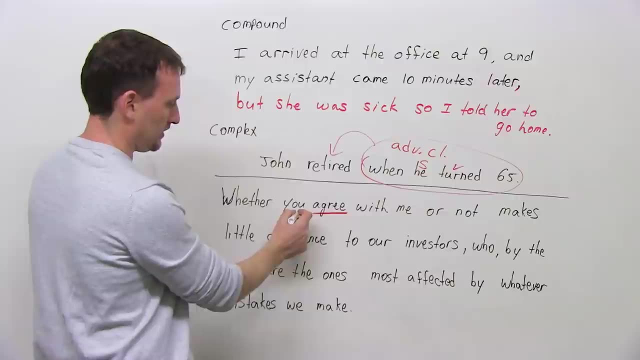 your independent clause is: first find your independent clause. Okay, Find your tense verbs: Any verb that has a past, present or future tense in any form. find that first. Agree. Okay, There's a subject to You, agree, This is one combination of subject verb. 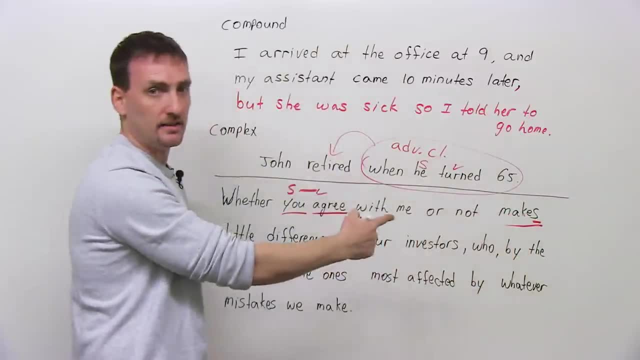 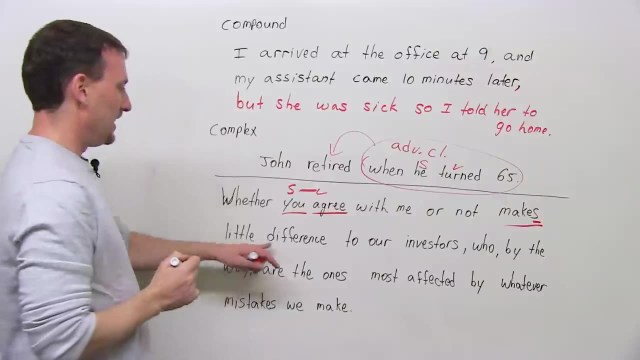 Or not. blah, blah, blah Makes. Well, that S tells you that this is a tense verb, Simple present. Okay, we'll figure out where the subject for it is All right, Little difference to our investors makes what. 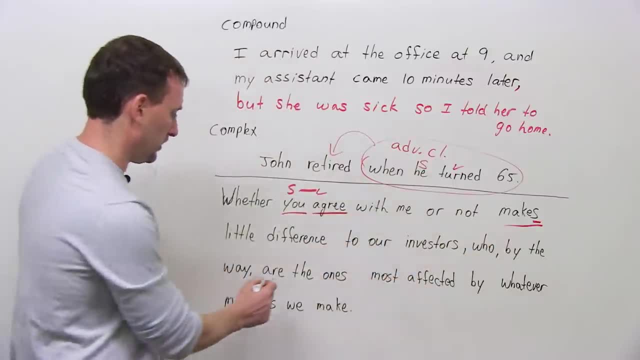 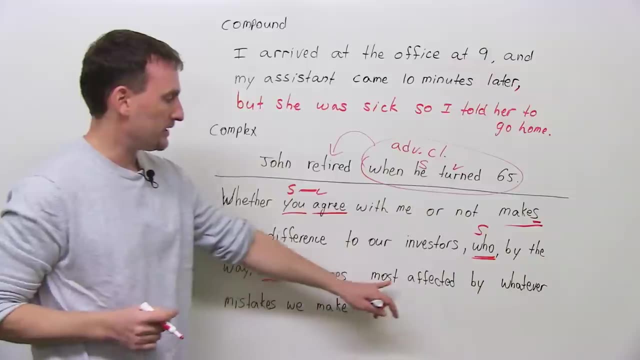 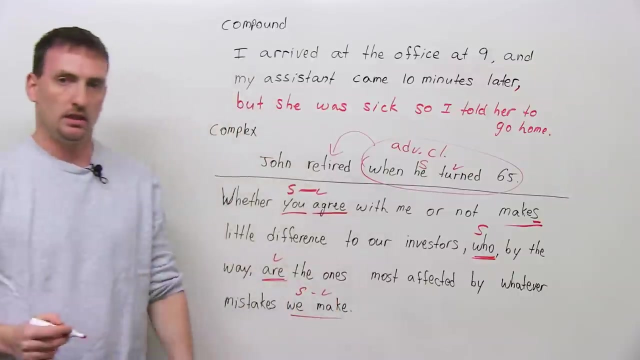 Who, By the way, are. So here's your Another tense verb And here's your subject for it. Okay, The ones most affected by whatever mistakes we make. And here's your last one. So now you're thinking: okay, well, I have subject verb, I have subject verb, I have. 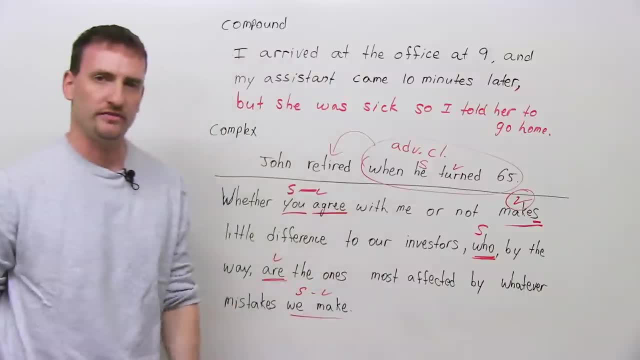 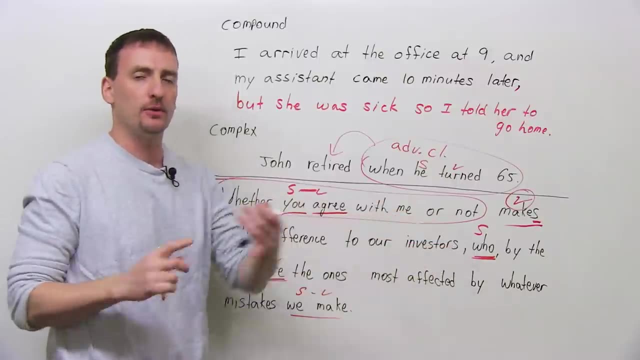 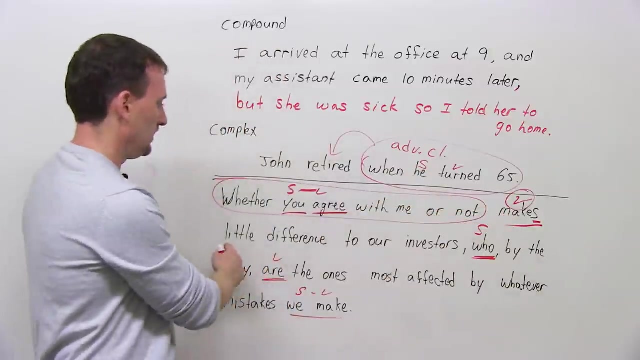 subject verb. Well, where is the verb? Where's the subject for this verb? And here it is Okay, This, This is a noun clause. Noun clauses act as subjects or objects. Okay, So this is your whole subject, This is your verb. Little difference to our investors. 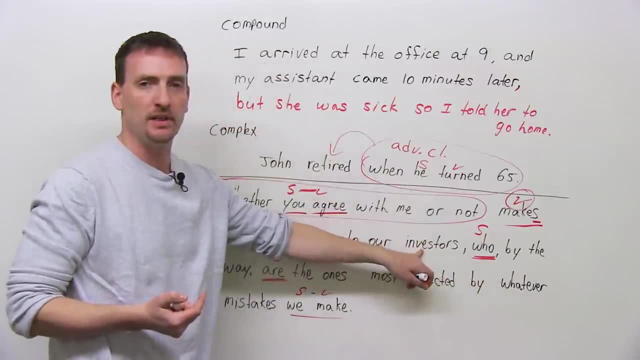 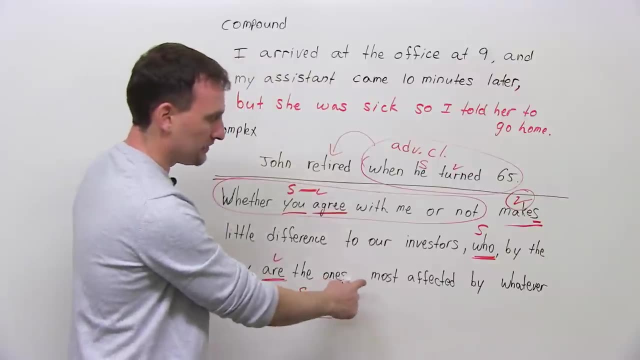 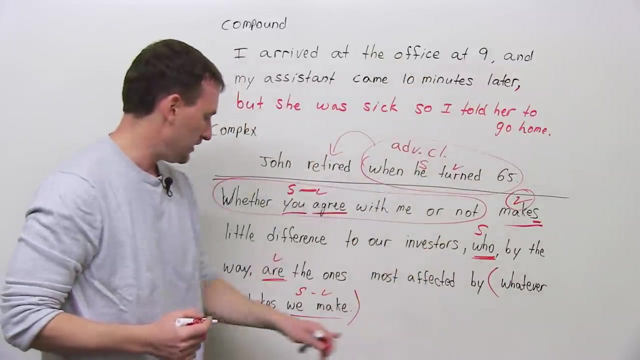 Now, here we have an adjective clause describing, Telling me something about investors, Telling me a little bit extra information about investors, Who are the ones most affected by By what- And here we have another noun clause: By what- And whatever mistakes we make. 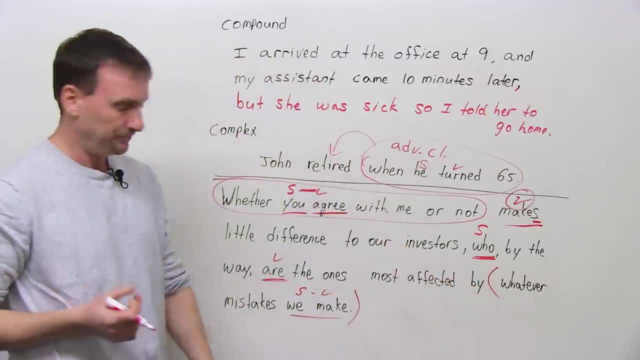 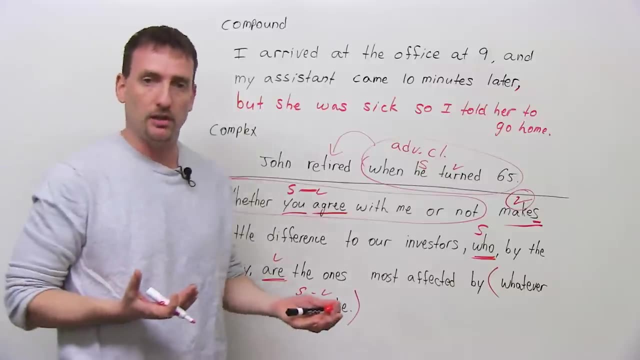 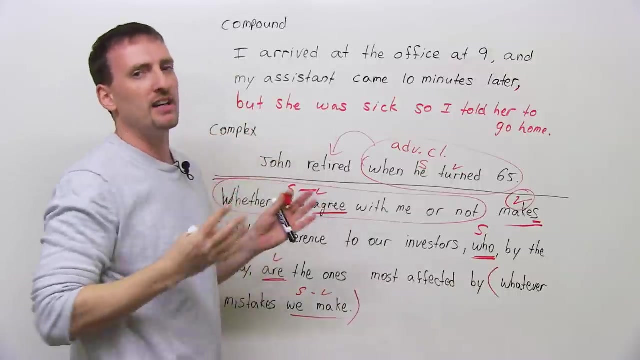 Whatever is the object? conjunction for mistakes. we make these mistakes. So now a little bit simpler, I hope. but you still see, I have my independent clause with a noun clause in it, which already makes it a complex sentence, but then I can add: 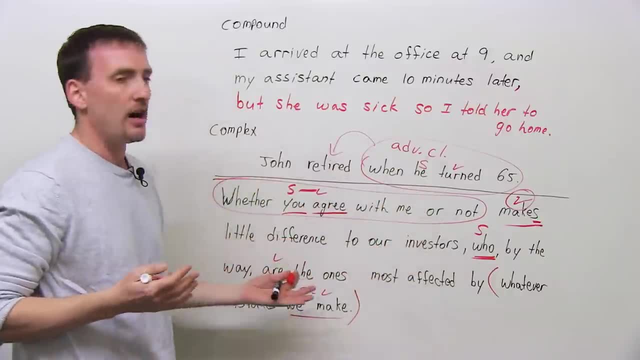 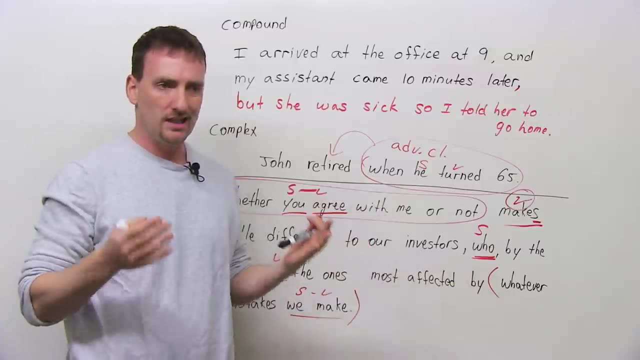 others. Okay, I can add as many as I need. This is not a bad sentence, but remember if it's getting out of control, if you're writing and your sentence is just too long, think about cutting it somewhere. Cut it in two, cut it in three, but make it very clear. 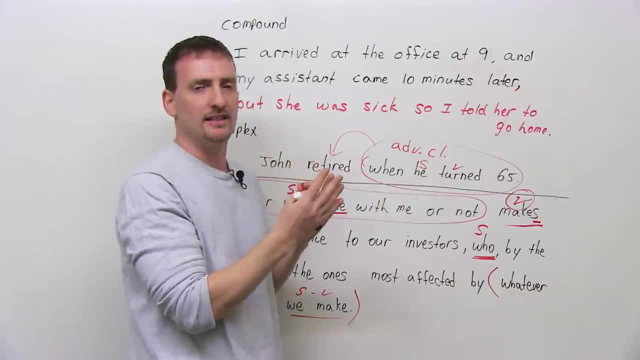 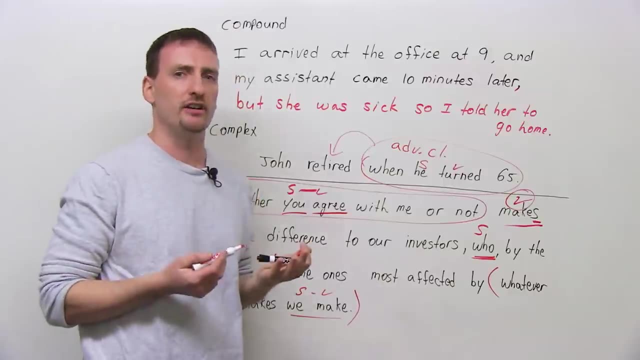 But at least keep one of the independent clauses in there so that you still have a complex sentence. Okay, Now we're going to look at the complex compound sentence. Now, these can be very tricky because you obviously have many clauses. You have to identify each one. 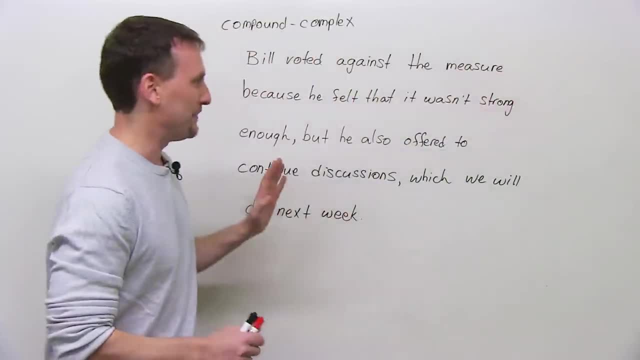 Let's look at an example. Okay, Let's look at our last example. Now, I know you're saying, I know you're thinking: oh, wait a minute, that's too short. It can't be that complicated, It's not. 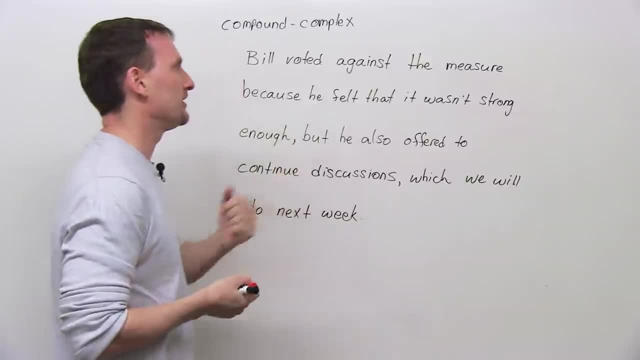 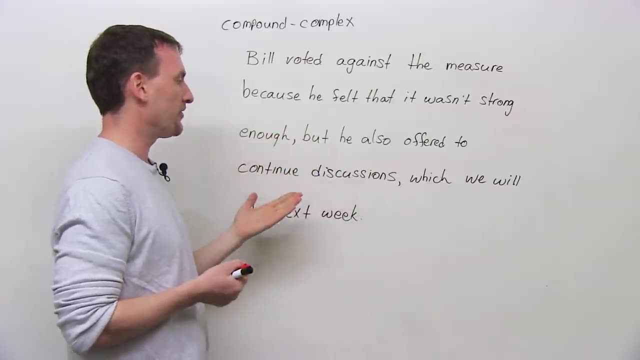 All the elements that should be there are there. First, let's read it. Bill voted against the measure because he felt that it wasn't strong enough, but he also offered to continue discussions, which we will do next week. Now, what do I have here? 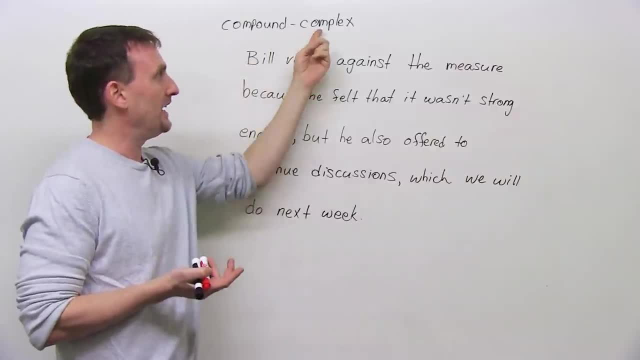 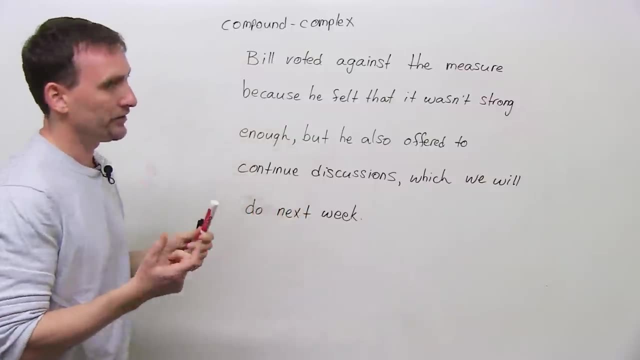 I have compound means, I have to have two independent clauses. and I have complex means, I have to have at least one dependent clauses. So let's look at First independent clause. Again, look for a verb, a tense verb voted. 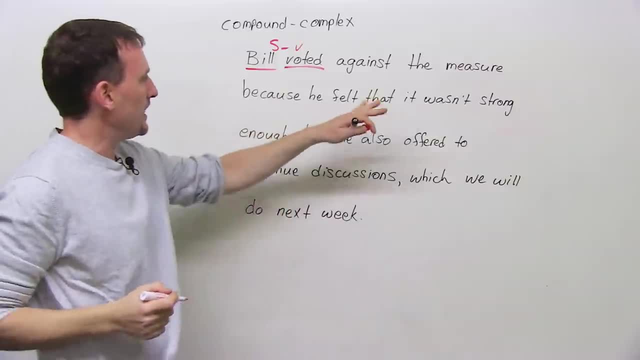 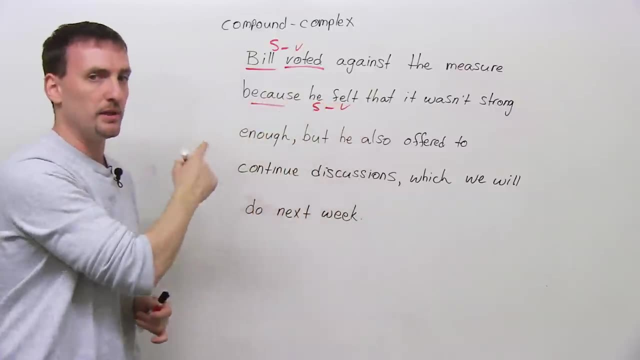 There's a subject bill, We have our subject verb Against the measure blah-blah, he felt. So here's a verb, here's another subject. but we know, because of the, because this is part of the dependent clause, it wasn't. 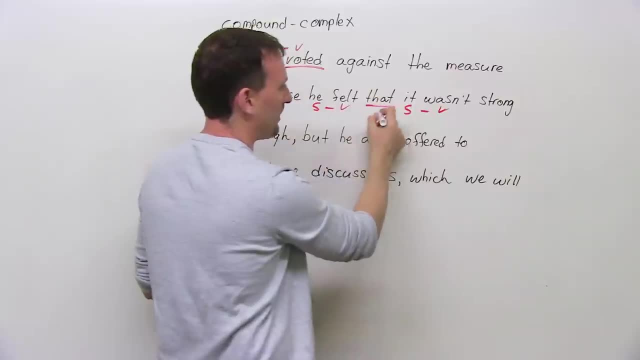 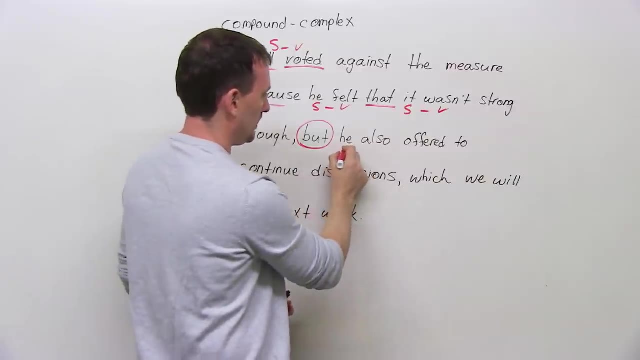 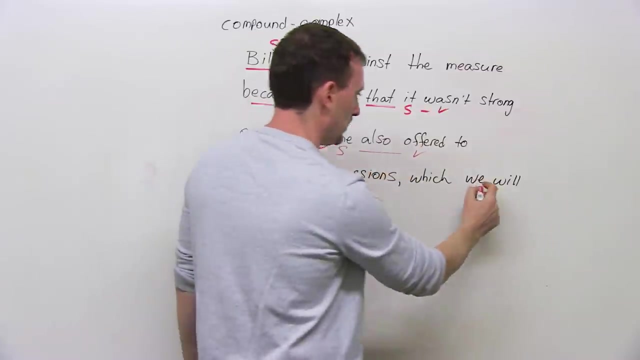 Okay, There, we have another verb, we have another subject, we have that, so that's another dependent clause. Oh, here's our conjunction. Okay, He Next subject offered. There's our: He offered to continue discussions, which we will do.